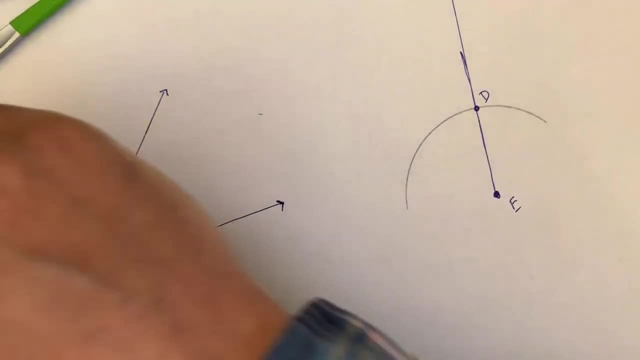 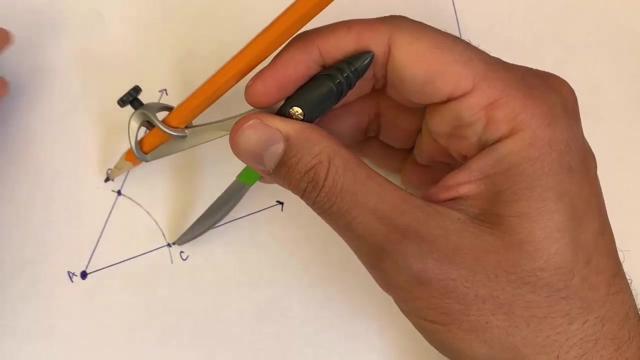 so that these two angles are congruent, And what I can do is take my compass again and get a clear sense of the distance between C and B by adjusting my compass. So one point is on C and my pencil is on B. 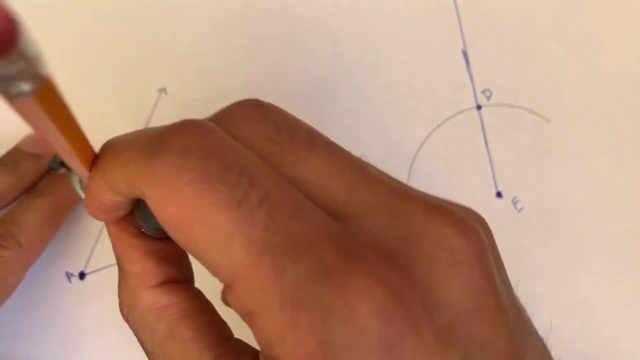 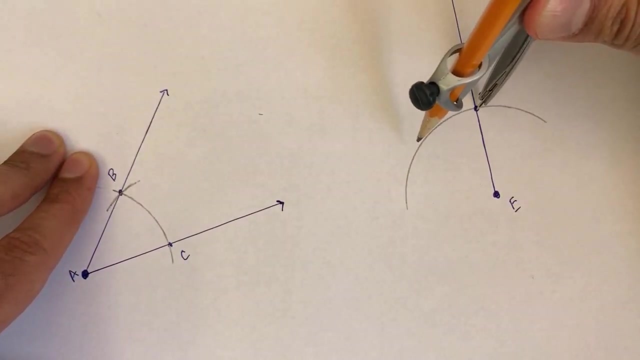 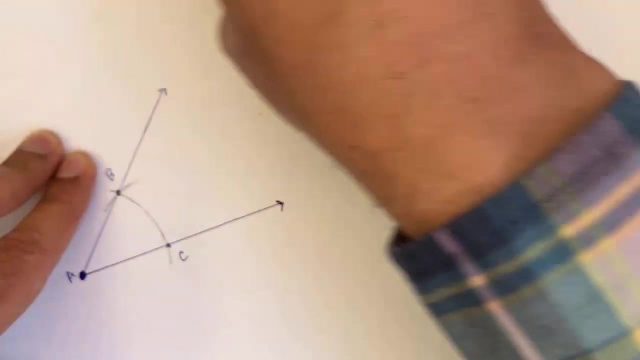 So I have let me get this right. so I have this distance right over here, I know this distance And I have adjusted my compass accordingly so I can get that same distance right over there, And so you can now imagine where I'm going to draw that second ray. 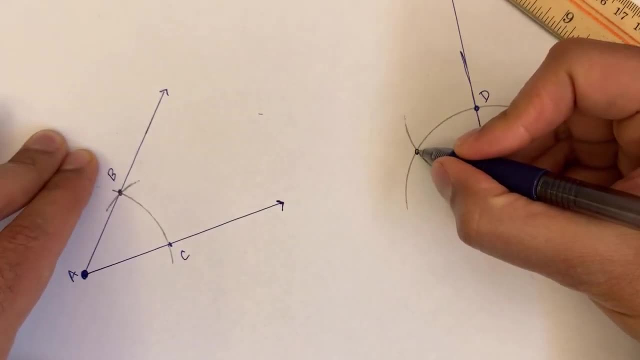 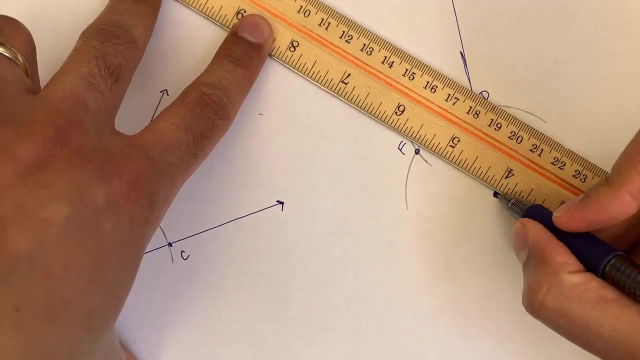 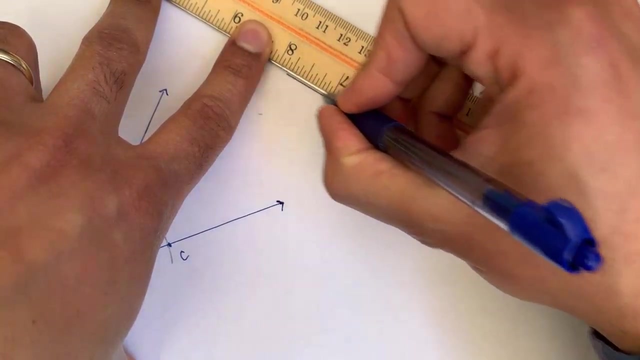 That second ray. if I put point F right over here, my second ray, I can just draw between starting at point E right over here, going through point F. I could draw that a little bit neater, So it would look like that. 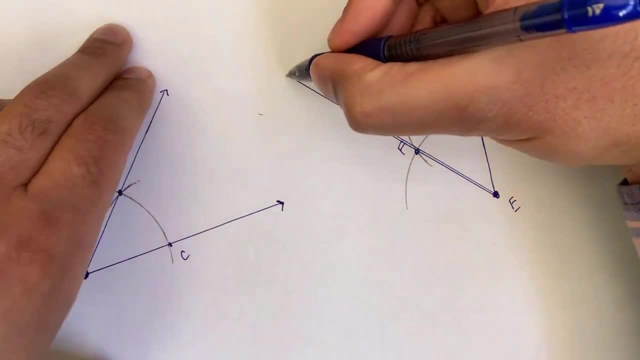 my second ray. Ignore that first little line I drew. I'm using a pen which I don't recommend for you to do it. I'm doing it so that you can see it on this video. Now, how do we know that this angle? 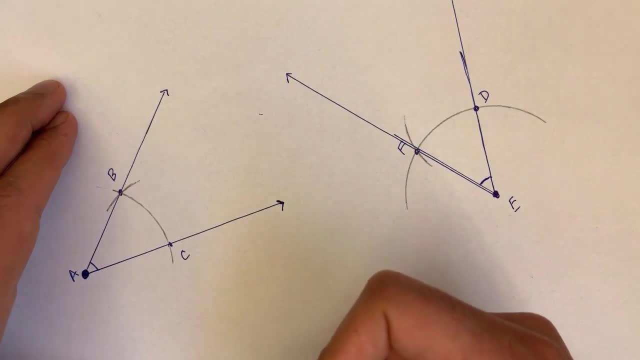 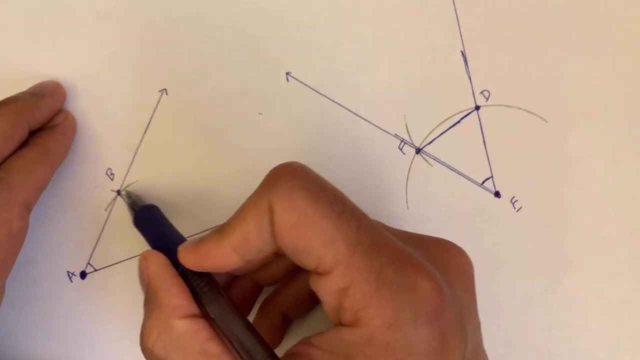 is now congruent to this angle right over here. Well, one way to do it is to think about triangle, BAC, triangle, BAC and triangle. let's just call it DFE, So this triangle right over here. When we drew that first line, 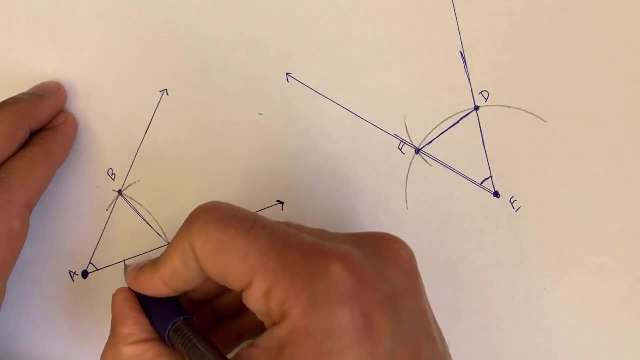 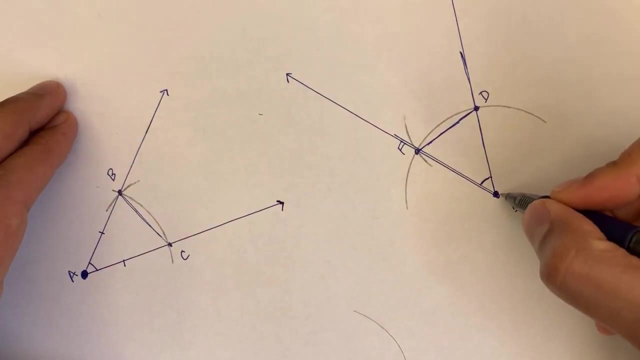 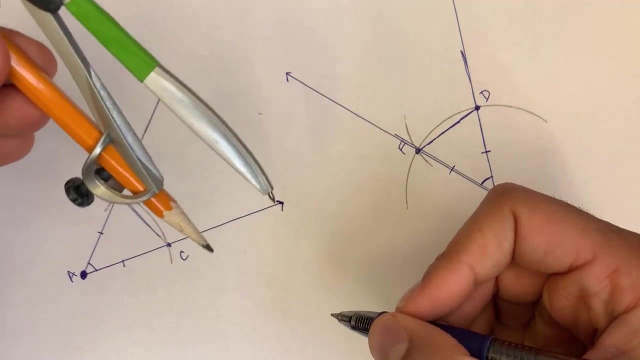 this first arc, we know that the distance between AC is equivalent to the distance between AB and we kept the compass radius the same. So we know that's also the distance between EF and the distance between ED. And then the second time, when we adjusted our compass radius, 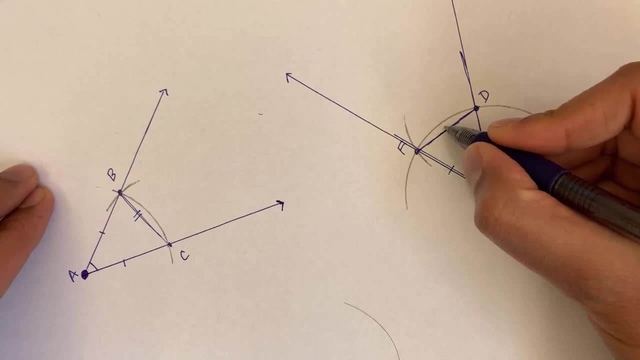 we now know that the distance between BC is the same as the distance between F and D, or the length of BC is the same as the length of FD. So it's very clear that we have congruent triangles. All of the three sides have the same measure. 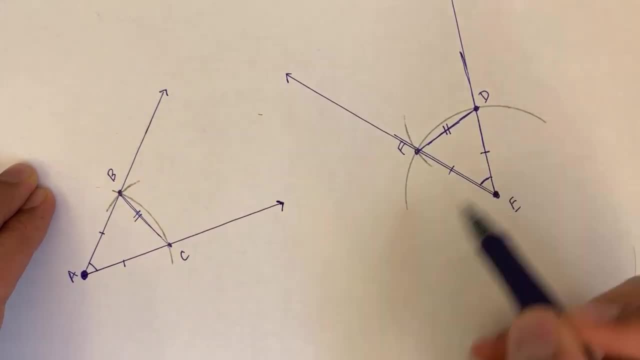 And therefore the corresponding angles must be congruent as well. the richest country in all of Europe by far is none other than Luxembourg. In fact, Luxembourg is the country with the highest GDP per capita on the planet. If we had to define Luxembourg's economy in one sentence, we could say that it is the country where unemployment does not exist and where one month's average salary is almost. enough to go on an all-inclusive year-long vacation in the Caribbean. To give you an idea, the average salary in Luxembourg is over $5,800 per month, And we are talking about the average salary. I don't even want to tell you what the most.